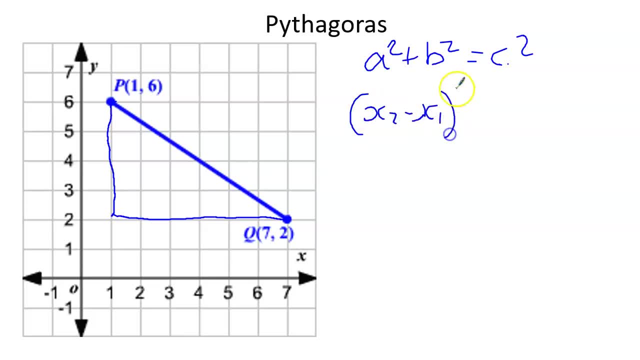 It would be: x2 minus x1 squared plus y2 minus y1 squared equals c squared, And of course we work that out and then we square root it. It doesn't actually matter which way around you subtract them, because we're going to square it. 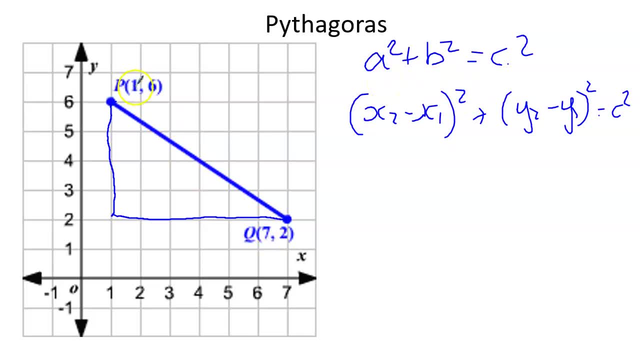 If you do the 7, take away the 1 and square it, or if you do the 1, take away the 7 and square it, you get the same amount. Okay, because one way you get 6 squared is 36.. 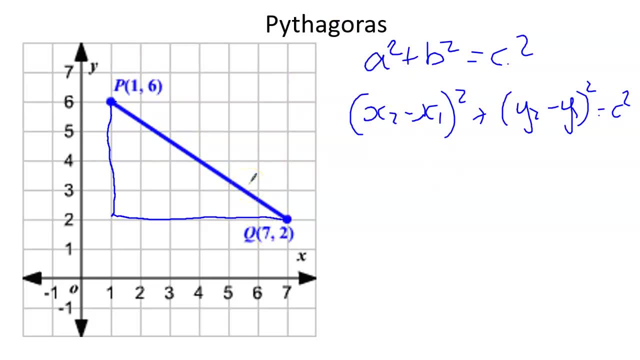 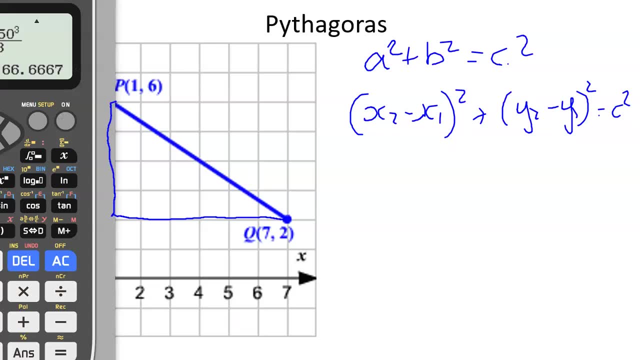 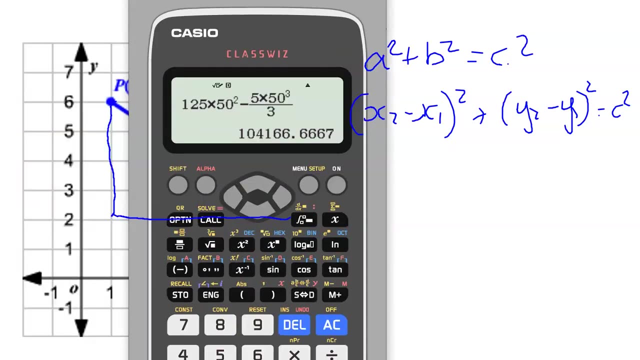 One way you get minus 6 squared is still 36.. But you've just got to be careful with your calculator, because if we get the calculator up on the screen, hang on, let's just change to a mouse instead of writing. If we get the calculator up on the screen and I type in minus 3 squared, 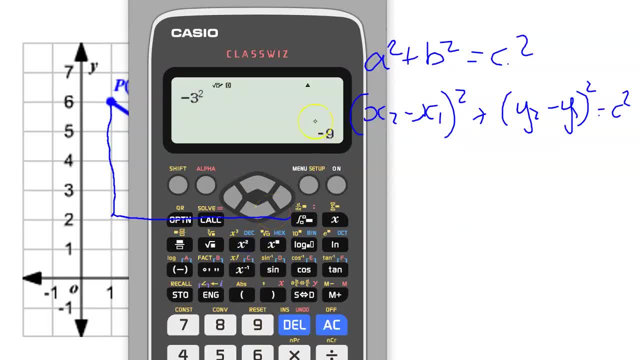 whoops minus 3 squared. then you see, it tells me minus 9, which is not the case. And the calculator's not wrong. It's because BidMath says to do the squared first. So make sure you pop a bracket round your squares and then it's not going to go wrong. 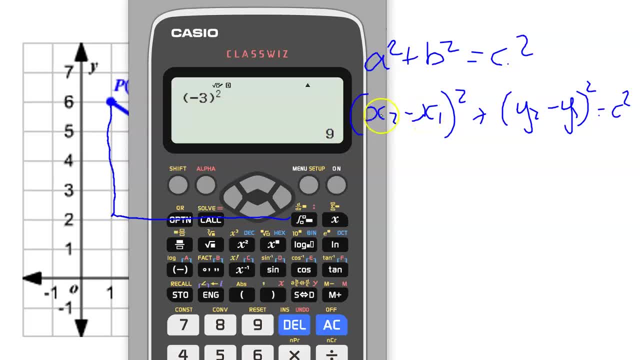 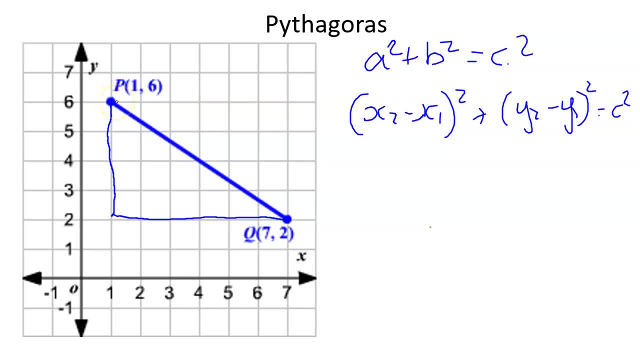 So just be careful. I would use brackets in this for sure, to make sure I didn't make silly mistakes with my minus signs. Anyway, back to the original problem. I want to work out this length, So I'm just going to work out the difference from 7 back to 1 and squared. 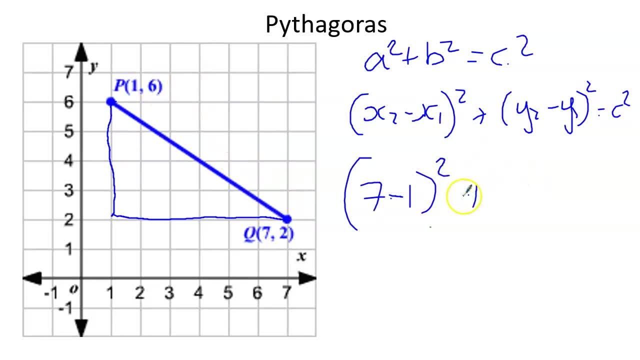 Plus from 2 back to 6,, which is minus 4 squared, and that equals C squared. So C, or the length of this line, is the square root of 6.. No 36.. I've got to square it. 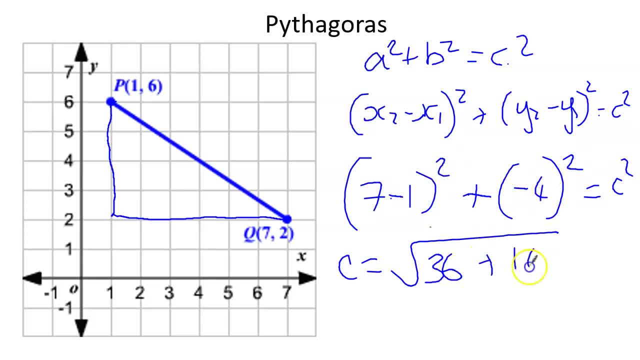 So that's 6 squared 36, and 4 squared is 16.. So this is the square root of what's that going to be? 52.. Which isn't going to be a nice number, unfortunately, but never mind. 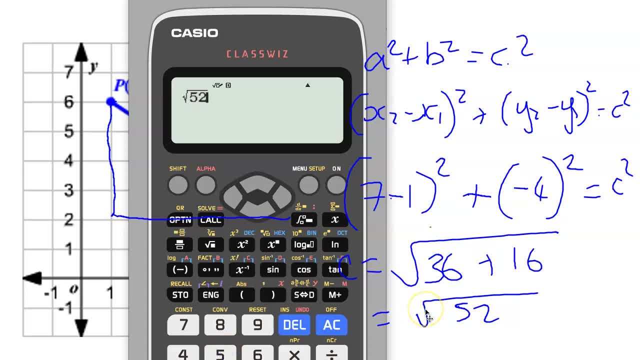 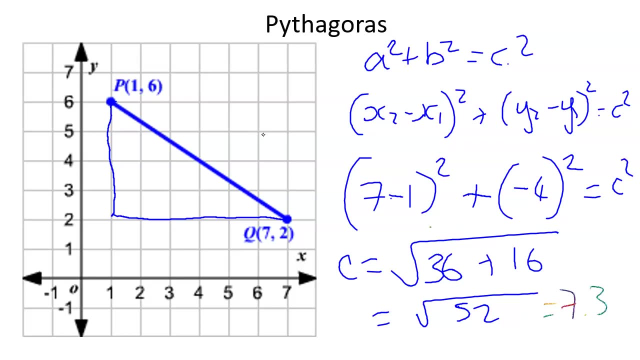 We can type that in The square root of 52 equals and press the SD button or the change button, and the answer is 7.21.. If in doubt, use three significant figures. Oh gone rainbow. What did we say?